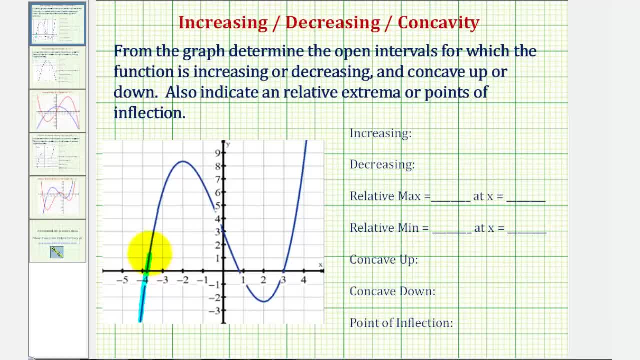 function is increasing over this interval until it reaches this high point. at x equals negative two. Also notice: if you were to sketch a tangent line at any point over this interval, the slope of the tangent line would be positive. But then notice from: x equals negative two. 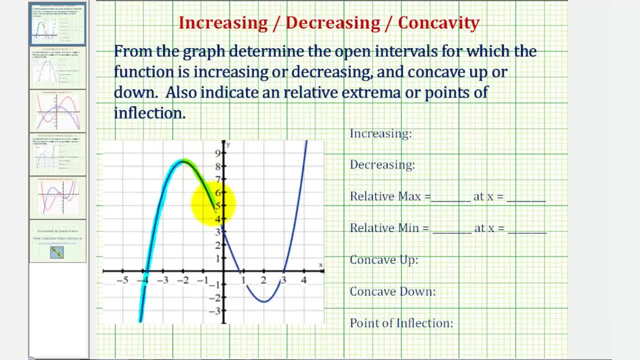 here to x equals positive two. the function is going downhill or decreasing until it reaches positive two here, and then it switches back to increasing from two to infinity. So notice how it changes from increasing to decreasing. at x equals negative two and it changes from decreasing. 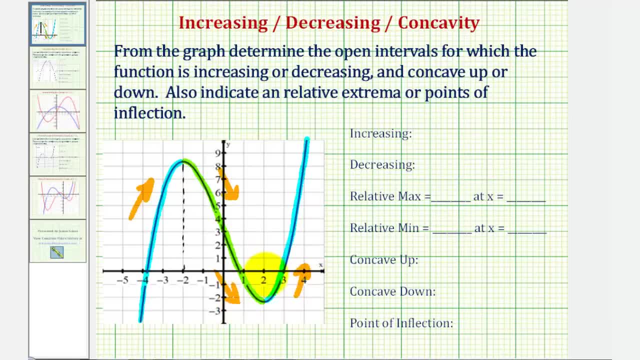 to increasing at x equals positive two And therefore the function is increasing over the open interval from negative infinity to negative two, but then it increases also on the open interval from two to infinity and it's decreasing over the open interval from negative two to positive two. 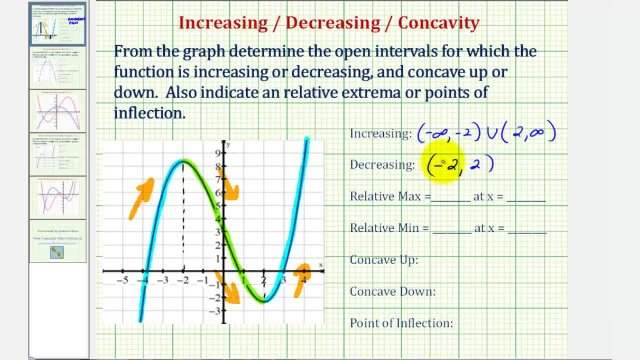 And notice: where the function changes from increasing to decreasing, we have a high point and therefore a relative maximum here, And where the function changes from decreasing to increasing, we have a low point or relative minimum. So the relative maximum values are the y values. 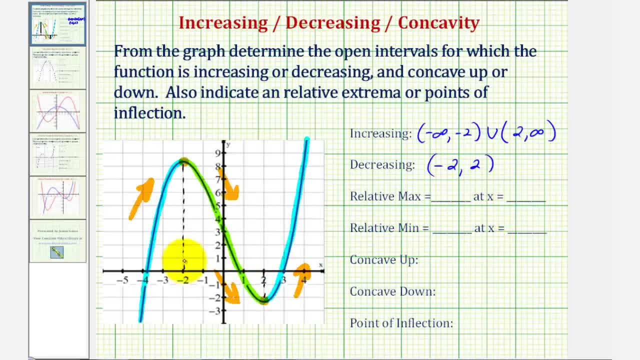 and the locations are the x values. So we can say we have a relative maximum of approximately, let's say, eight. point three: at x equals negative two. sometimes you'll see the relative maximums given as ordered pairs as well. and then we have a relative minimum of, let's say, x equals negative two, point three. 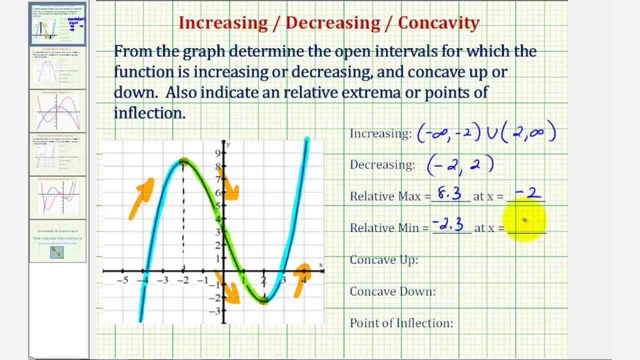 at x equals positive two. And now let's talk about the concavity. Looking at the left side of the graph, notice how this piece is concave down, and it seemed to change concavity right at the y-axis. Now, on the right, the function is concave up. 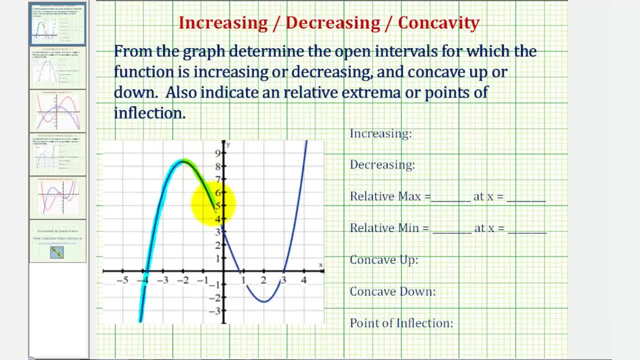 here to x equals positive two. the function is going downhill or decreasing until it reaches positive two here, and then it switches back to increasing from two to infinity. So notice how it changes from increasing to decreasing. at x equals negative two and it changes from decreasing. 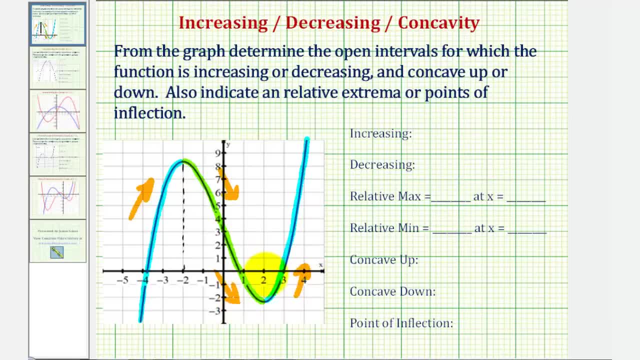 to increasing at x equals positive two And therefore the function is increasing over the open interval from negative infinity to negative two, but then it increases also on the open interval from two to infinity and it's decreasing over the open interval from negative two to positive two. 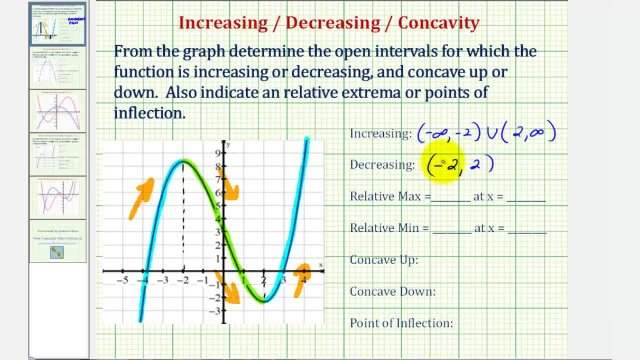 And notice: where the function changes from increasing to decreasing, we have a high point and therefore a relative maximum here, And where the function changes from decreasing to increasing, we have a low point or relative minimum. So the relative maximum values are the y values. 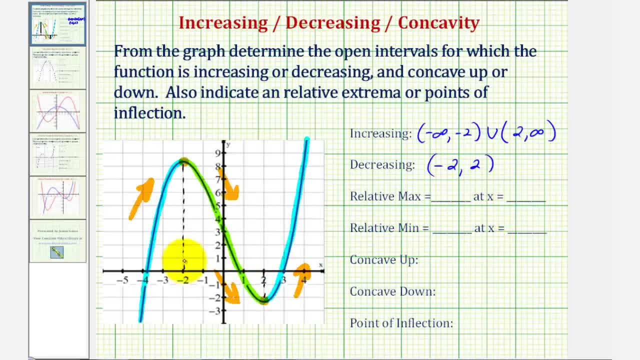 and the locations are the x values. So we can say we have a relative maximum of approximately, let's say, eight. point three: at x equals negative two. sometimes you'll see the relative maximums given as ordered pairs as well. and then we have a relative minimum of, let's say, x equals negative two, point three. 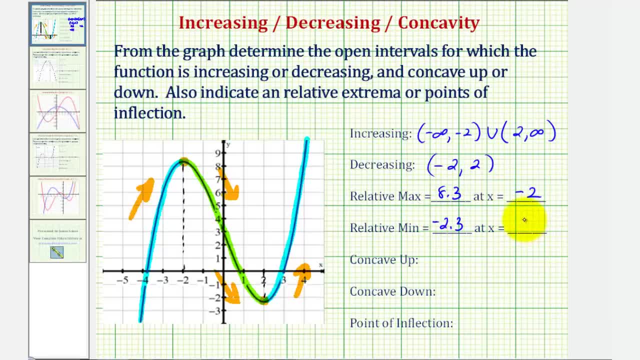 at x equals positive two. And now let's talk about the concavity. Looking at the left side of the graph, notice how this piece is concave down and it seemed to change concavity right at the y-axis And on the right the function is concave. 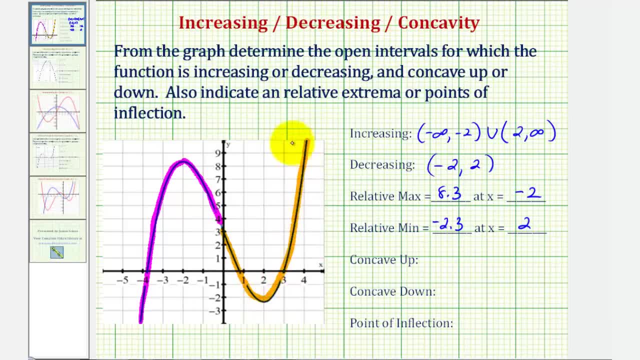 up. So on the left the function is concave down and on the right the function is concave up. Again we're going to say it changes concavity right at x equals zero or this point here. So we can say the function is concave up.